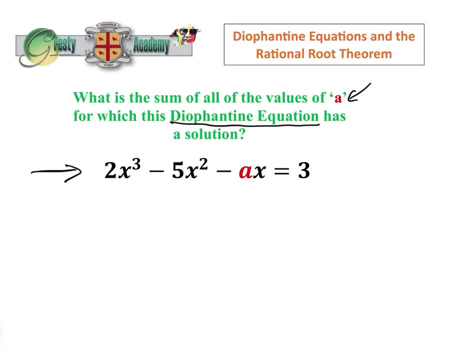 has a solution. Okay, so here's the Diophantine equation, and what they're saying is whether it has a solution. what they mean is: does it have an integer solution? Okay, so what we're going to do is- we are clearly because of this title- here we're going to use the rational root theorem. 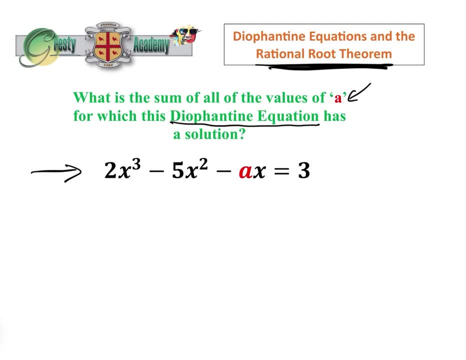 Now what the rational root theorem says is that if we have a polynomial c n, x to the n and c n minus 1, x to the n minus 1, add c 0 equals 0.. If all of the coefficients are integers, ie all of. 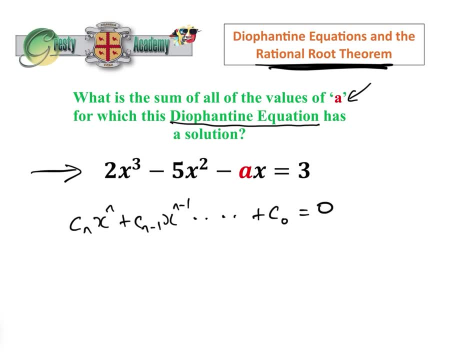 the c are integers, and if there is a rational solution, let's call it p over q, where p and q are co-prime, ie we have got rid of all of the common factors of p and q. Then p is an integer factor of c 0 and q is an integer factor of c n, ie p divides c 0 and q divides c n. Now we're. 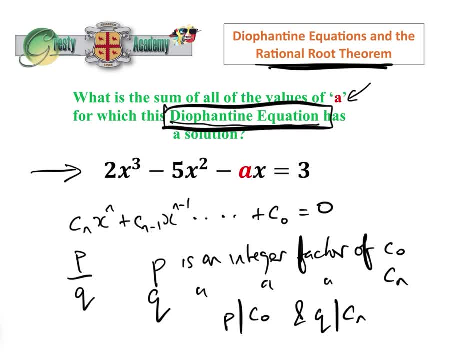 not looking for rational solutions here because we're told this is a Diophantine equation. so we're only looking for integer solutions Now. an integer therefore. by definition q is going to be 1, so we can ignore that part of the rational root theorem and this part and all. 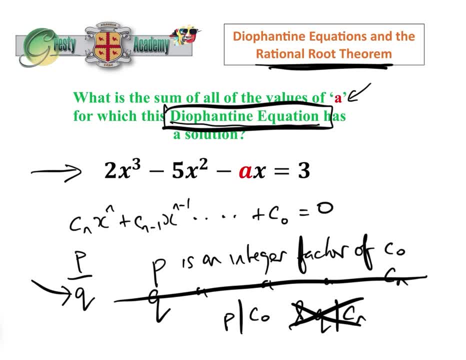 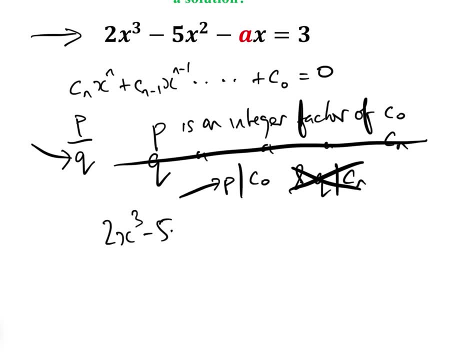 we're left with is that, in order to have an integer solution, p must divide c 0.. So let's just rewrite our question: 2 x cubed minus 5, x squared minus a x as minus 3 equals 0, and then we have: 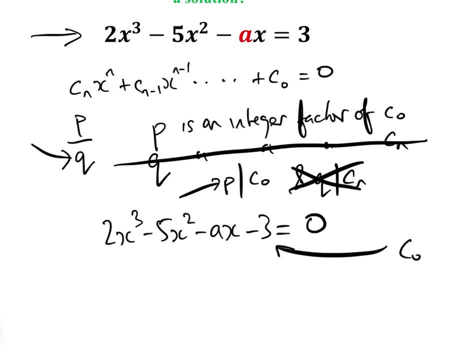 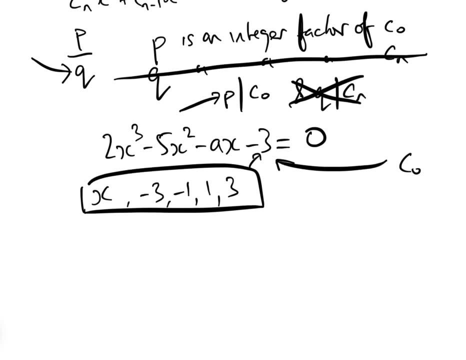 here our c 0 in our polynomial is minus 3, and so therefore, by the rational root theorem we know that we can only be minus 3, minus 1, 1 or 3, which are the four factors of minus 3.. So all we need to. 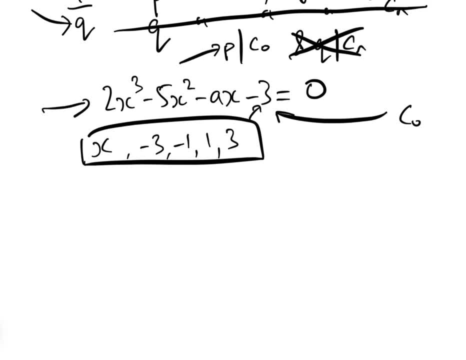 do now is stick each of these values into our equation and find out what the value of a must be. So let's say, when x is minus 3, we know that is a solution because of the rational root theorem. Then we got minus 5. so all I'm doing now is I'm sticking minus 3 into here, so that gives us minus.